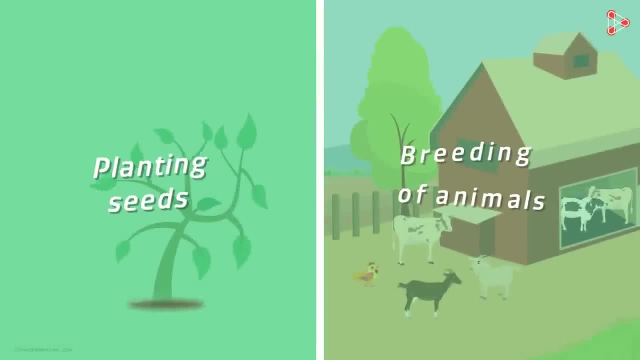 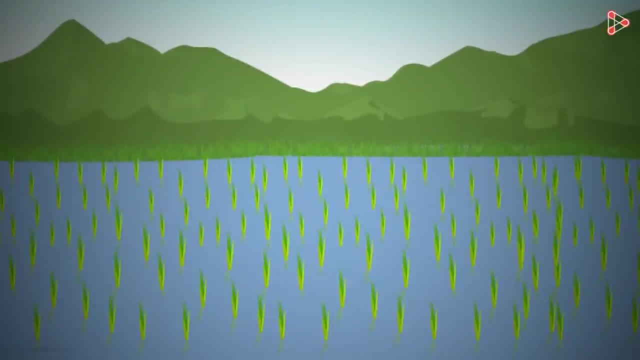 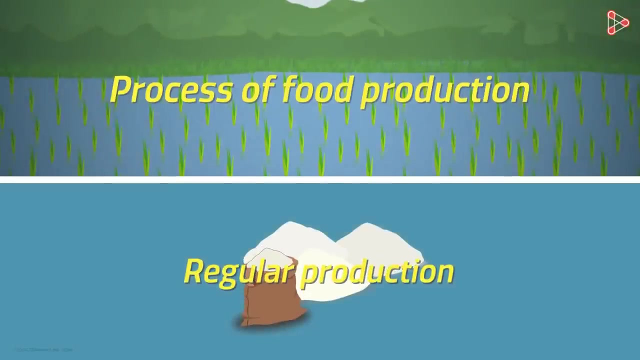 What do we mean by producing food? Are planting seeds and breeding of animals the only events in food production? Of course not. A lot of effort goes into the process, The process of food production. One of the things this process includes is regular production of food. 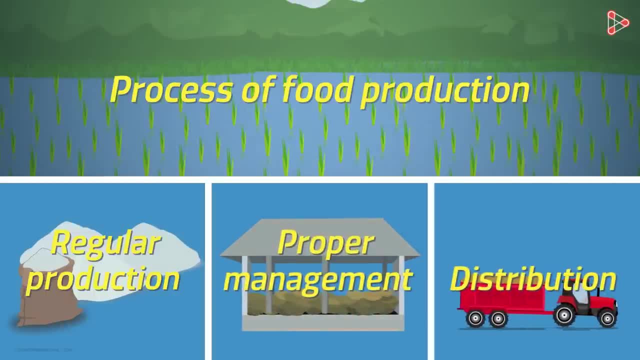 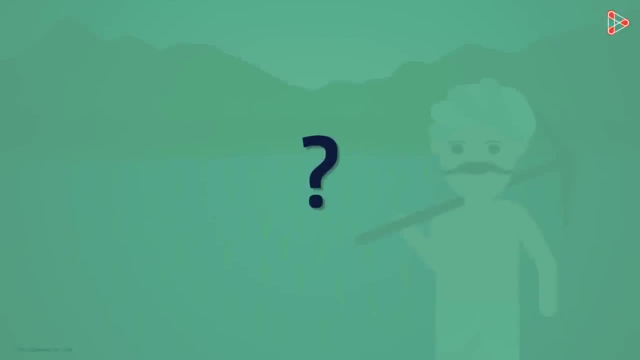 Secondly, proper management of the resources produced And lastly, fair distribution among the people. But how did this idea of food production come into existence? What do we call production of plants in a specific area of land, Agriculture? You guessed it right. 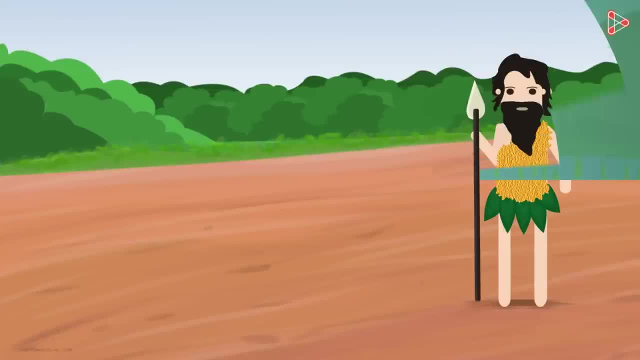 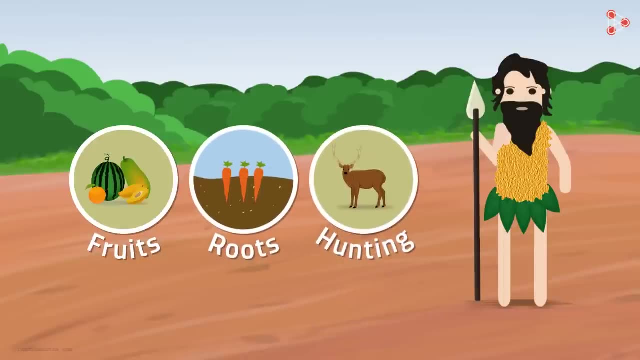 But how did man get this idea of agriculture? How did man get this idea of agriculture? This idea of agriculture has been problematic for many years. Survival was mainly dependent on fruits, roots and hunting of animals for food. Eventually, man learnt the culture of cultivation. 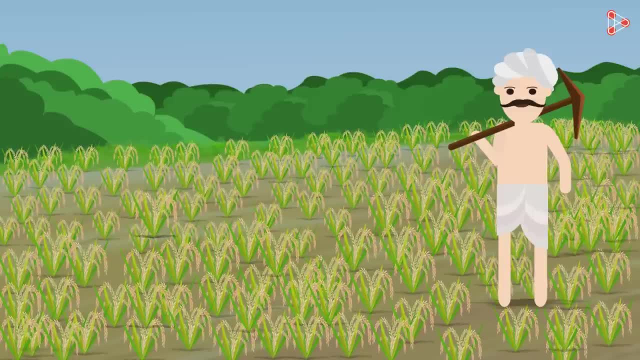 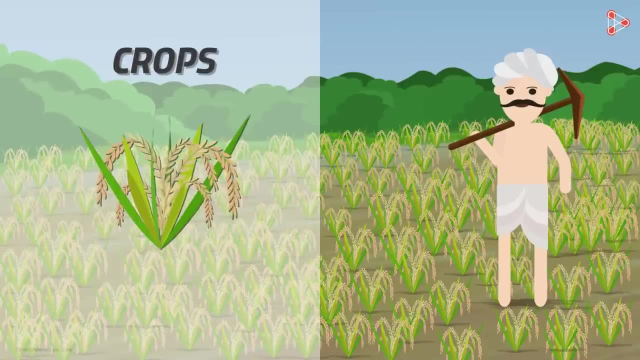 Man learnt agriculture by observing nature. So what is the most important part among all the components in agriculture? Of course the crops. But what exactly do we mean by crops? When seeds of a plant are grown on a large scale, we call it a crop. 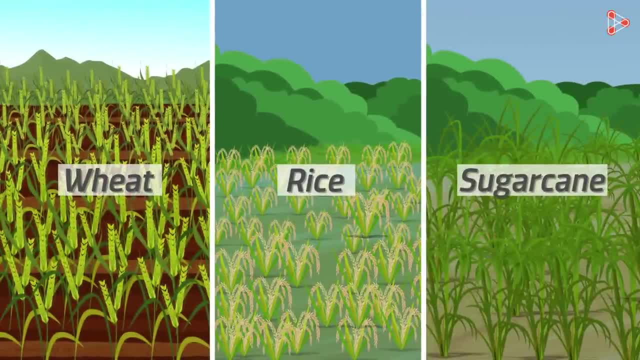 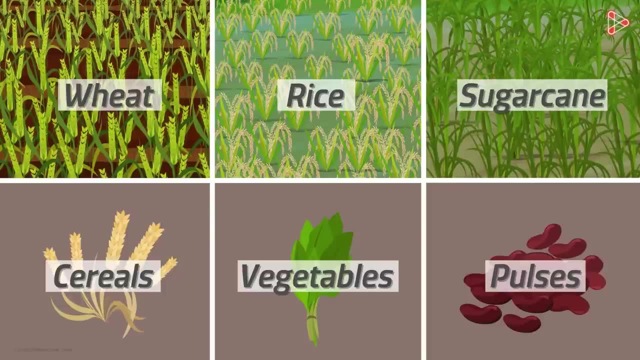 Crops of wheat, rice or sugarcane can be grown at a time on a piece of land. Crops can be of cereals, vegetables or pulses, but each crop needs a specific type of weather. Crops are therefore classified based on the season they are grown in. Can you guess which two types of crops are grown in India? Let me help you with that. The two major crop seasons in India are the season of the Karif crops and that of the Rabi crops. What is the difference between the two? 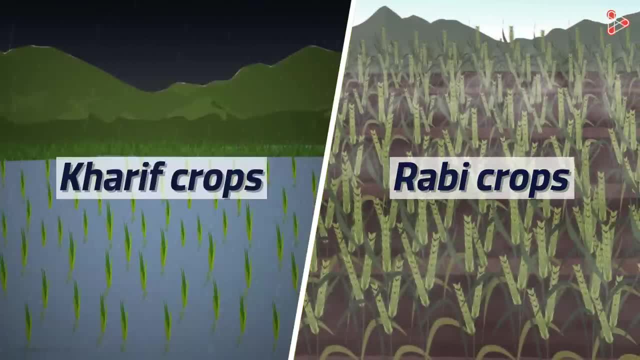 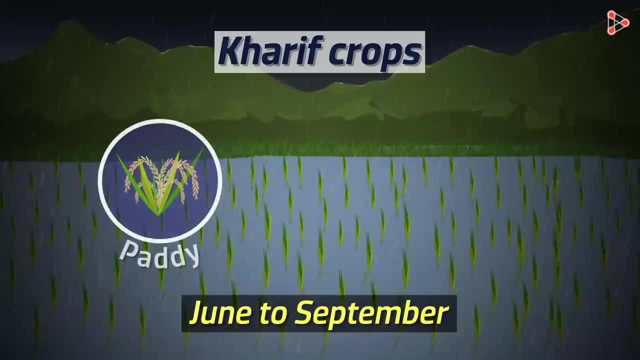 The former are sown in the rainy season, while the latter are sown in the winter season. Rainy season in India spans from June to September. Crops grown in this period are paddy, maize, soybean, which require moisture and a large quantity of water. 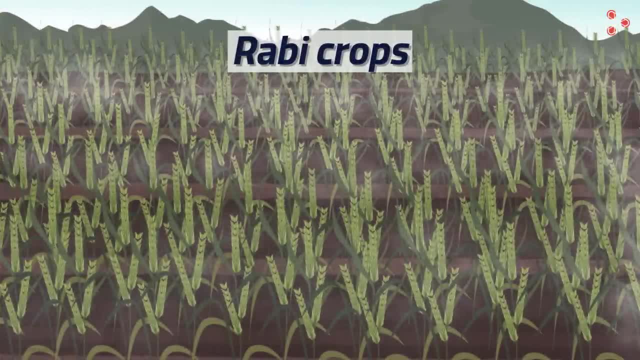 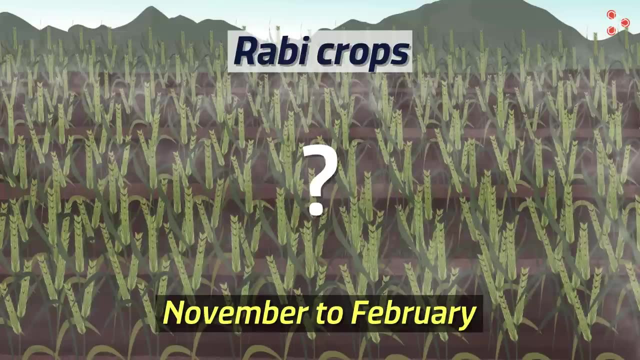 When does India have winter? Winter months in India begin with the month of November, extending till the month of February. Which crops do you think are best suited in this climate? Take a guess: Yes, wheat, mustard and grams are a few of the winter crops. 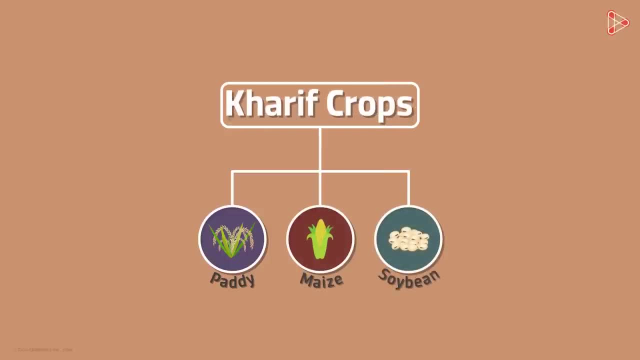 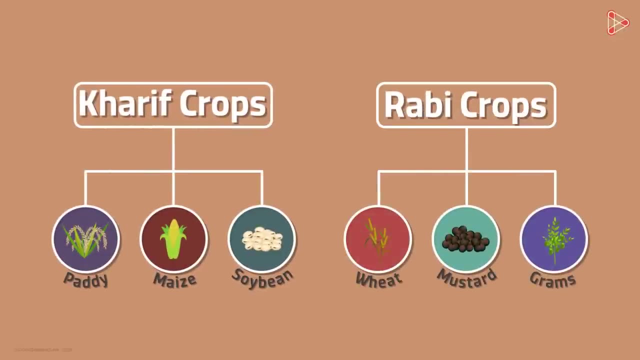 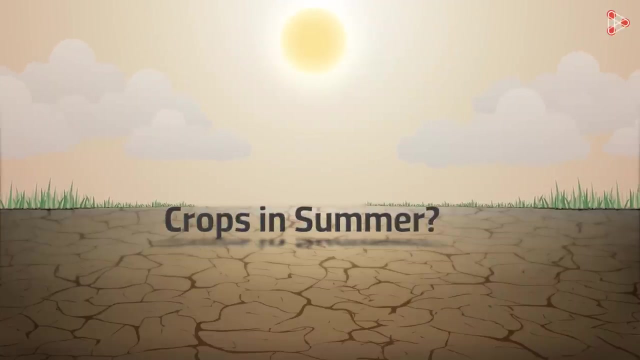 So can we say that paddy, maize and soybean are Karif crops? Yes, And similarly we can say that wheat, mustard and grams are Rabi crops. What is grown in the summer months, then? Well, summer months usually do not see a lot of cultivation.